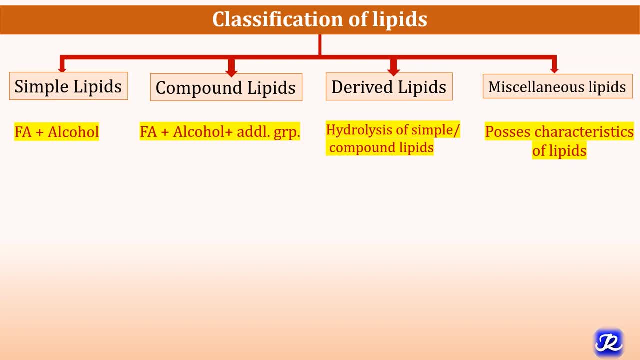 and miscellaneous lipids are those which do not fall in any category of simple, compound and derived, but they possess the characteristics of lipids. What are simple lipids? They are the lipids with various alcohol. The examples of simple lipids are triacylglycerol or triglyceride. 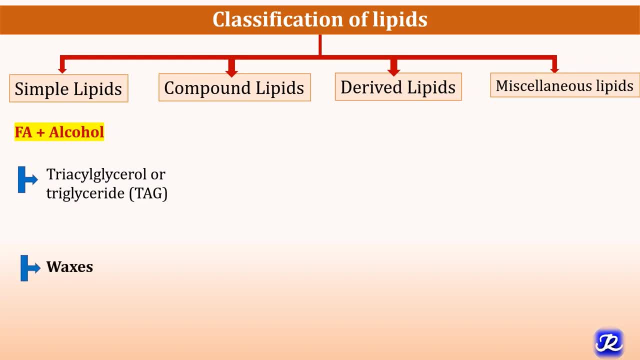 which is also called as TAG and waxes. TAG are the stirs of fatty acid with glycerol and they are uncharged. that's why they are also called as neutral fat. The fat we mostly eat is triacylglycerol, and fat that is deposited in our body as a fuel source that is also triacylglycerol. 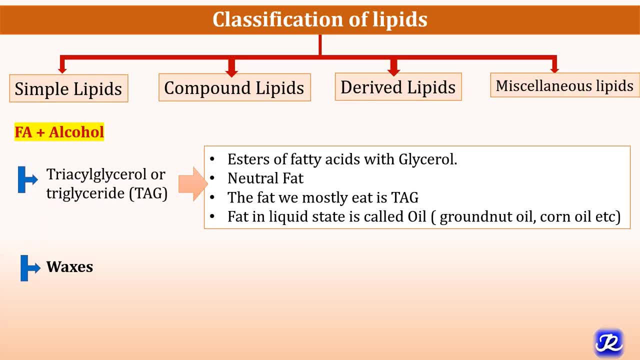 Fat in the liquid state is called oil. for example, the vegetable oils like groundnut oil, corn oil, etc. And the waxes are stirs of fatty acids with high molecular weight, monohydric long-chain alcohol, and they are not important in human metabolism but they are widely used. 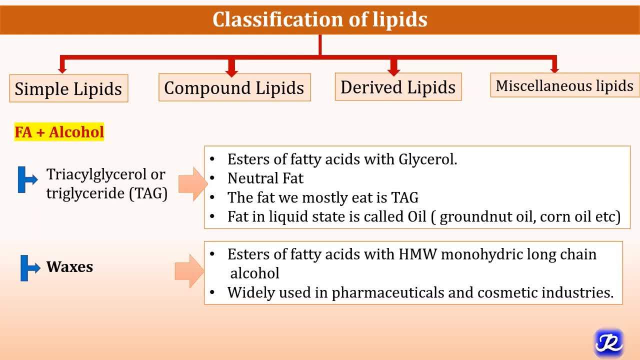 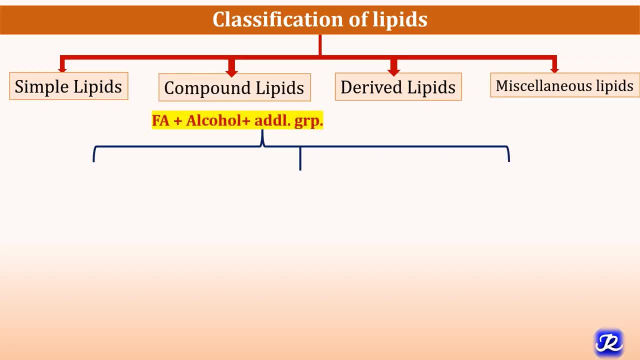 in pharmaceuticals and cosmetic industries to make certain lotions and ointments. Compound lipids are made up of fatty acids plus alcohol. The examples are phospholipids, glycolipids, lipoproteins. Phospholipids consist of fatty 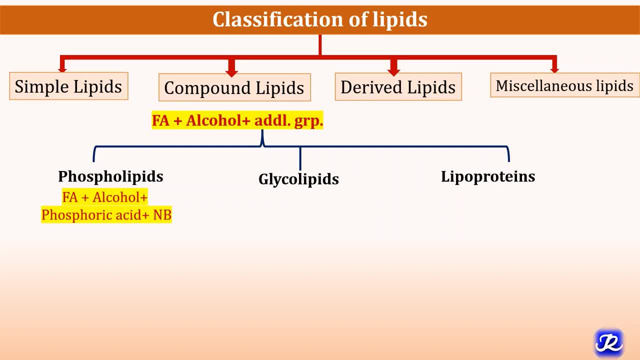 acid plus alcohol plus phosphoric acid and nitrogenous base, And depending on the type of alcohol present in the phospholipid, they are further classified as glycerophospholipid if the alcohol is glycerol and sphingophospholipid if the alcohol present is sphingosine. 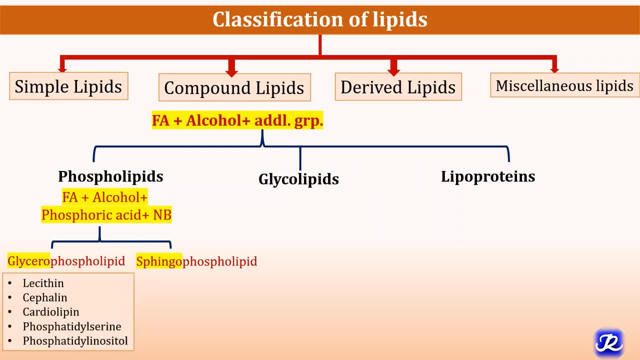 Zinc, billsol, hieratopsin, bunkerτil, choline, cephaline, cardiolipin, phosphatidylserine, phosphatidy, Portland, Zukinee, phosphatidylinositol, plasmalogen. These are the example of glycerphospholipid. 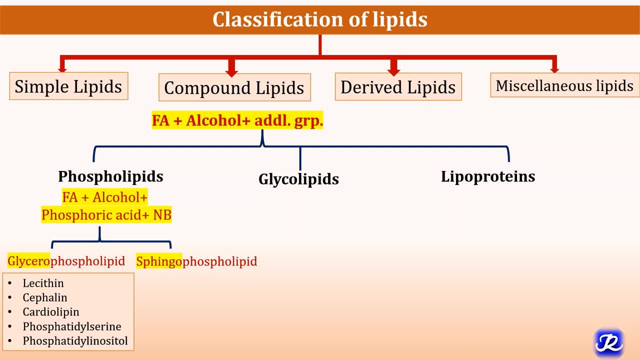 which neighbor lycerol as alcohol And sphingomylin contains, matched with sphingosine in the example of sphingophospholipid. Glycolipids consist of fatty acid plus alcohol and carbohydrates。 Carbohydrates are the glycol lipids. Carbohydrates consist of glycol lipid. 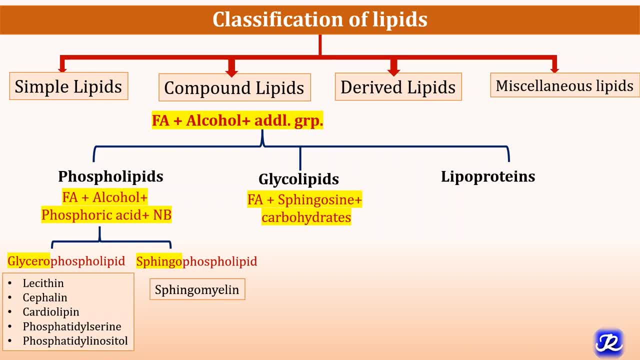 Gluc 진, glycol lipid, that is all are present in glycerol, plus alcohol, plus carrots. That's why they are called glycol lipid. Carbohydrates are known by our term glycol lipid, as it contains lipid and carbalanced lipid. 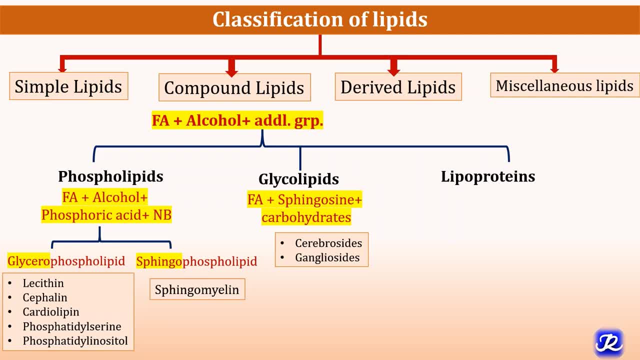 lipids. The examples are cerebrosites and gangliosites. The third example is lipoproteins, which are complex molecules made up of lipid plus protein, and the examples are chylomicrons. very low density lipoprotein, that is VLDL. low density lipoprotein, that is LDL, and high density. 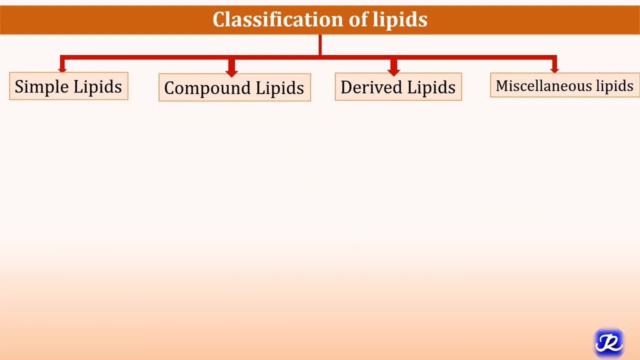 lipoprotein, that is, HDL. The third class of lipid is derived lipids, and these lipids are obtained on hydrolysis of simple and compound lipids. The examples are fatty acids, steroids which contain steroid hormones like mineralocorticoid, glucocorticoid, estrogen, progesterone. 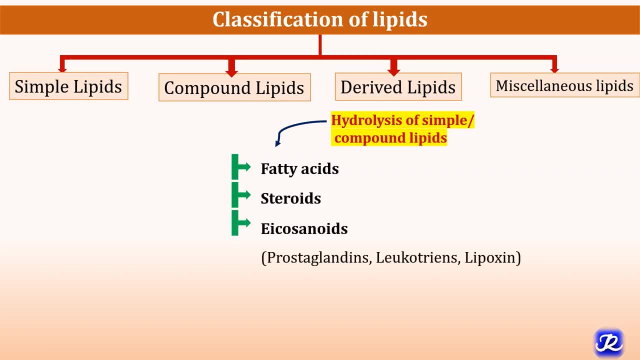 testosterone, etc. Ecosanoids which are derived from arachidonic acid, which are 20 carbon compound, and the examples are prostaglandins, leukotrienes, lipoxines, Ketone bodies. are also derived lipids which are formed from acetyl-CoA. 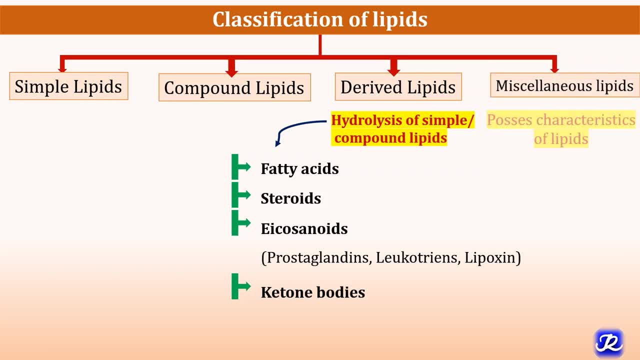 The fourth class of lipids is lipoproteins. The third class of lipids is lipoproteins. The fourth class of lipids is miscellaneous lipid and they possess the characteristics of lipids, for example, squalene, which is formed during the synthesis of cholesterol, and carotenoids. 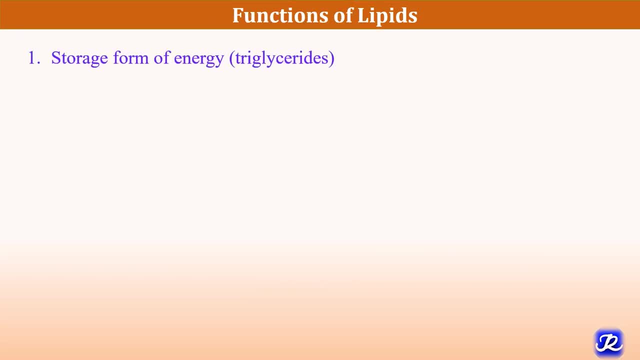 Let's enumerate the functions of lipids. They are the storage form of energy. Triacylglycerol are stored in the adipose tissue and in fasting and starvation adipose tissue. triacylglycerol are broken down to form fatty acids which are further oxidized for energy. 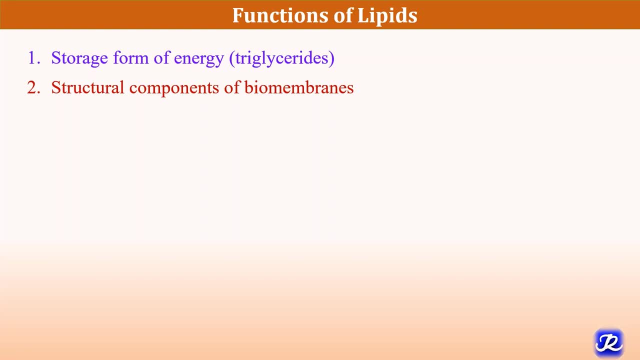 They are structural component of biomembranes, For example, phospholipid and cholesterol. they are present in cell membrane. Metabolic regulators like steroid hormones, ecosanoids like prostaglandins and leukotrienes perform various functions in the body. They act as surfactants, detergents and 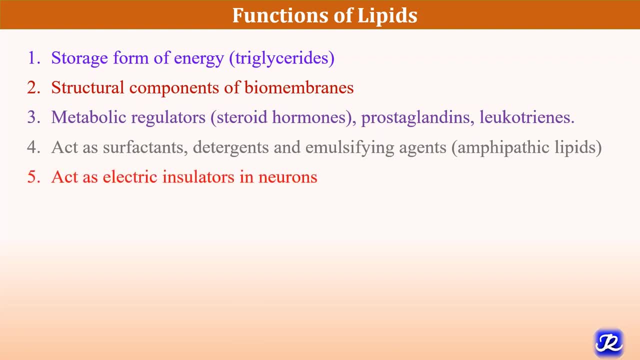 emulsifying agents Also act as electrical insulators in neuron, for example sphingomyelin. They provide insulation against changes in external temperature due to subcutaneous fat. They give shape and counter to the body. They protect the internal organs due to pairs of fat.